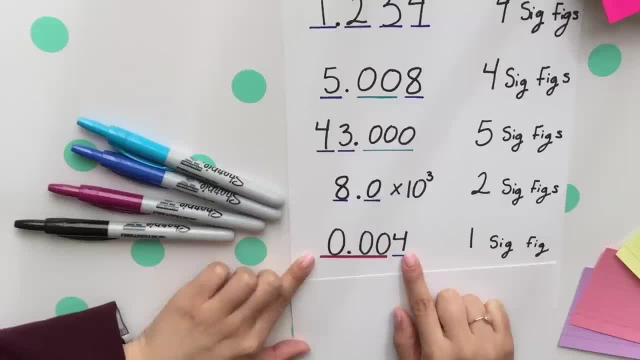 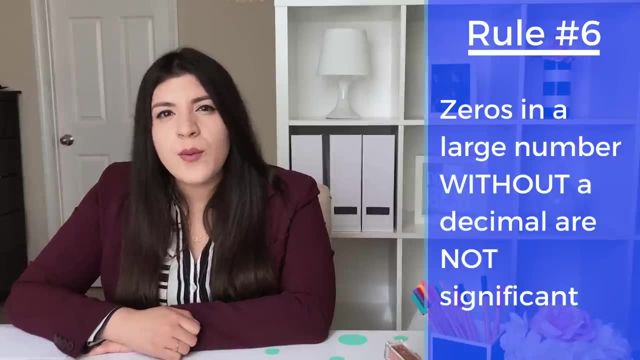 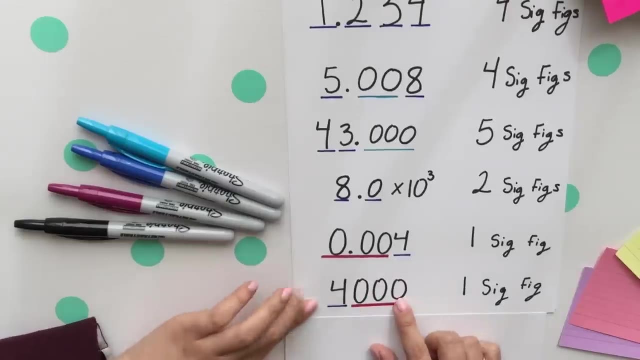 They do not count as significant. Only this four counts. so there's only one sig. fig. Rule number six: any zeros in a large number without a decimal are not significant. These three zeros are within a large number without a decimal, so they do not count as significant, Only the four. 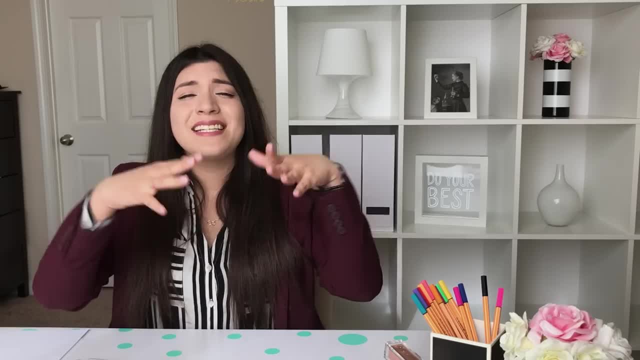 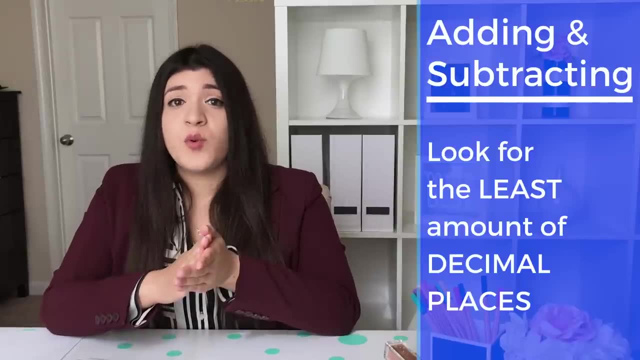 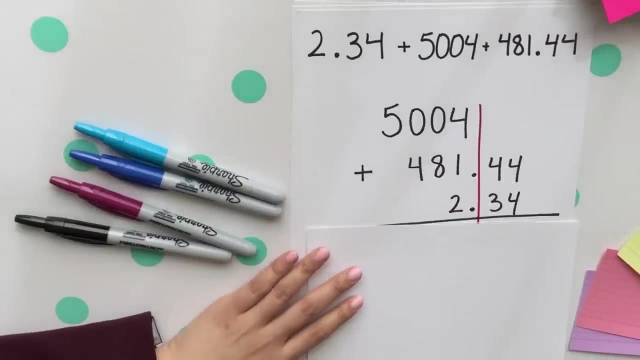 does. There's only one sig fig. All right, there's more. When adding and subtracting numbers, you look for the least amount of decimal places. For this first example, your first step is to line up all the decimal places. Notice how. 5,004, there is no decimal, However, where the decimal would be would be. 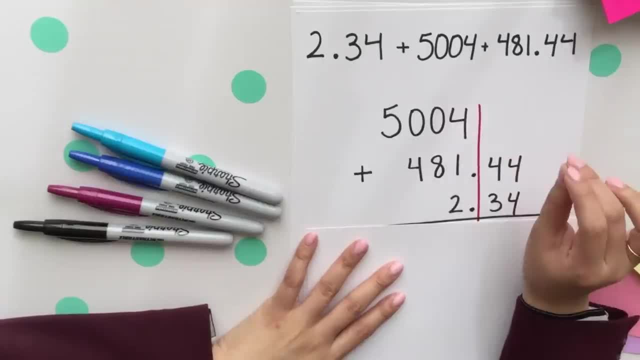 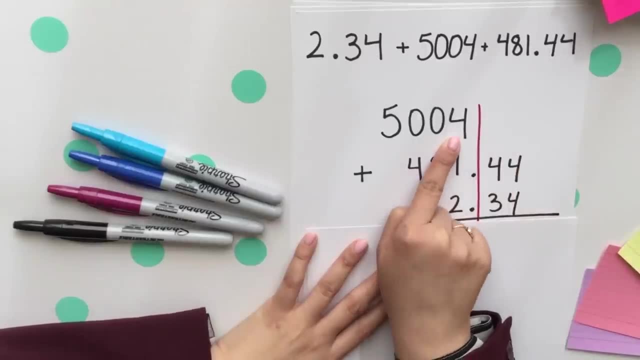 after this, four in the ones place. So since we're looking for the least amount of decimal places, that 5,004 doesn't have a decimal place, so we will round to the ones place. Remember, when rounding to the ones place or rounding any number, 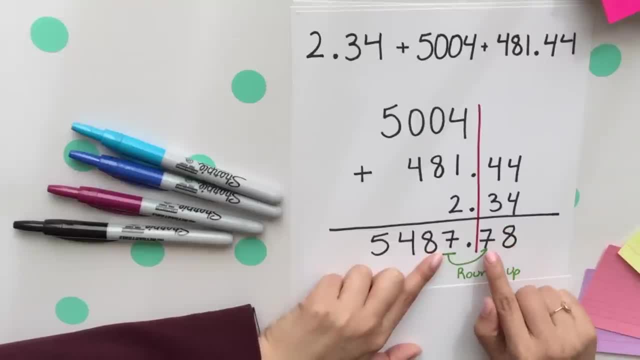 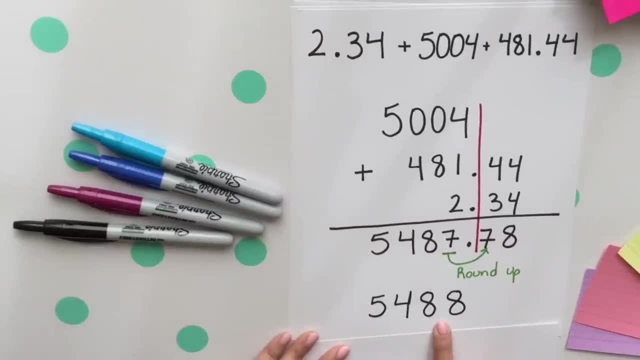 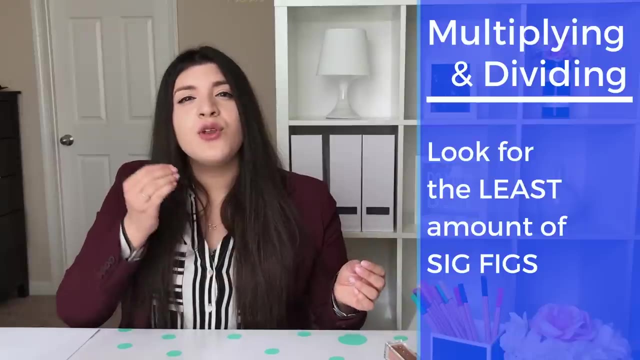 you look at the one right next to it, to the right, And if it is five or more, you round up. Your final answer will be rounded up to 5,488.. We have four sig figs. Moving on to multiplication and division, When multiplying and dividing you look for: 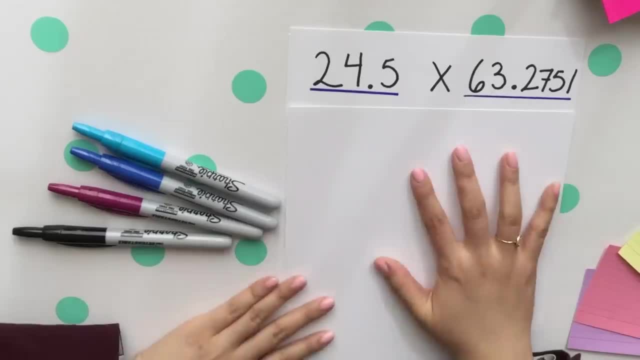 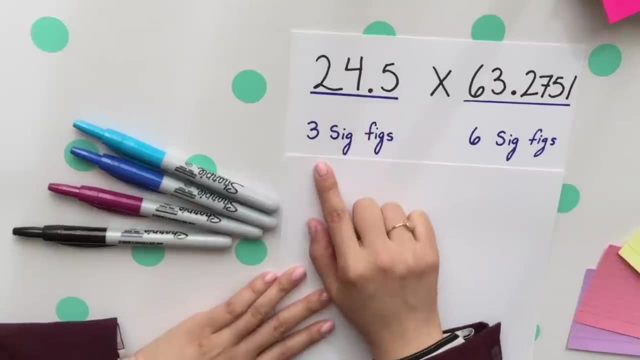 the least amount of sig figs. Your first step is to figure out how many sig figs did you there are within each number. Notice that there are three sig figs in this first number and six sig figs in the second. So we will round to three sig figs After. 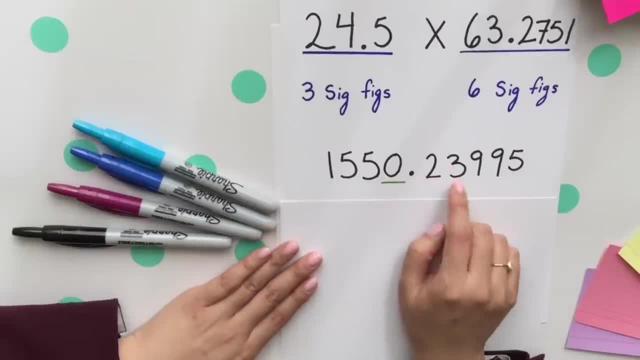 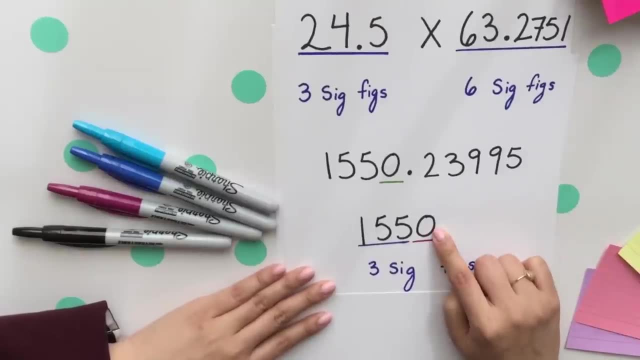 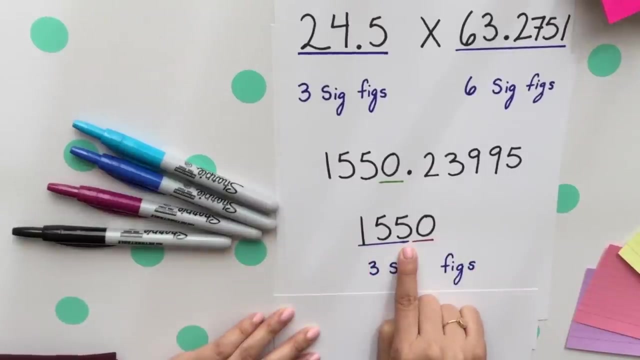 multiplying. you then want to go ahead and stop at this zero. so you remove that decimal place and there really only are three sig figs. because of that last rule, this zero does not count. there is no decimal place. it's within a large number. only these three count as sig figs. It's time to check yourself. Go ahead and try.